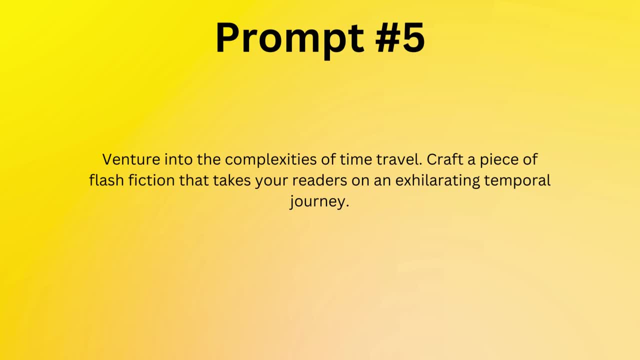 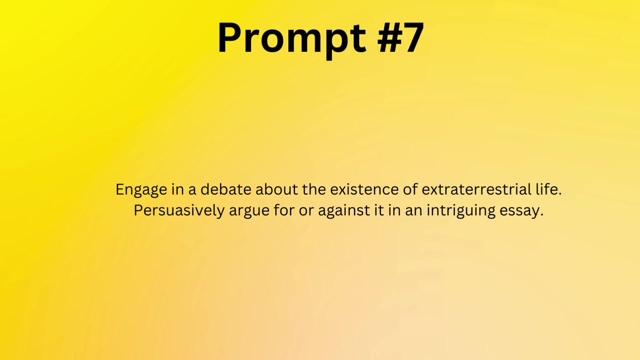 of time travel Craft, a piece of flash fiction that takes your readers on an exhilarating temporal journey. Prompt number six: Imagine a world where animals can communicate with humans. Write a captivating dialogue between a person and their beloved pet. Prompt number seven: Engage in a debate about the existence of extraterrestrial life, Persuasively argue for or against it in an intriguing essay. 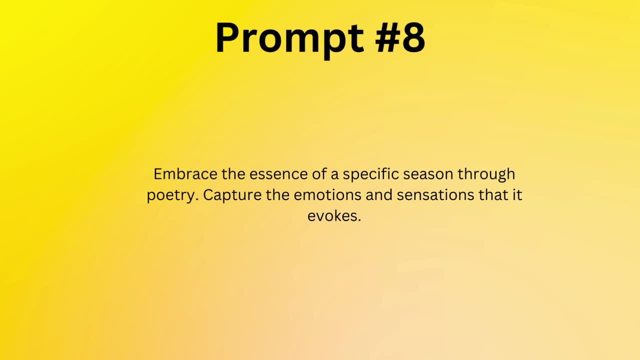 Prompt number eight: Embrace the essence of a specific season through poetry. Capture the emotions and sensations that it evokes. Prompt number nine: Find inspiration in visual art Craft: a short story based on a painting or photograph that ignites your imagination. 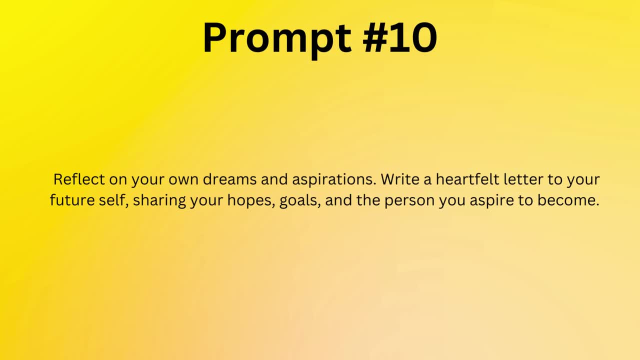 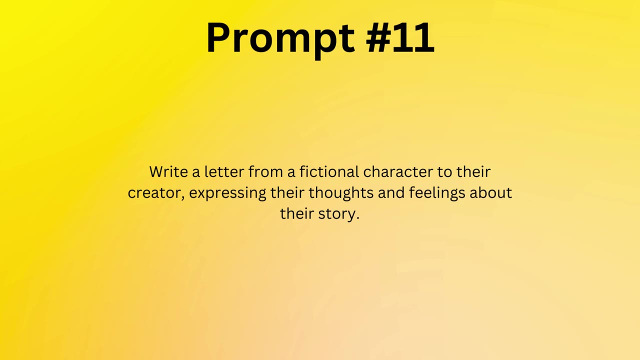 Prompt number ten: Reflect on your own dreams and aspirations. Write a heartfelt letter to your future self, sharing your hopes, goals and the person you aspire to become. Prompt number eleven: Write a letter from a fictional character to their creator, expressing their thoughts and feelings about their story. 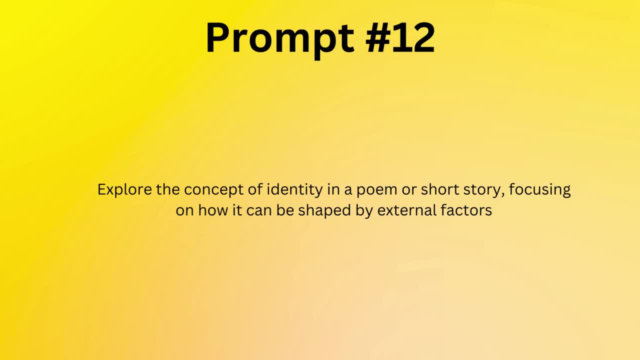 Prompt number twelve: Explore the concept of identity in a poem or short story, focusing on how it can be shaped by external factors. Prompt number thirteen: Create a dialogue between two inanimate objects, giving them personalities and allowing them to engage in a conversation. 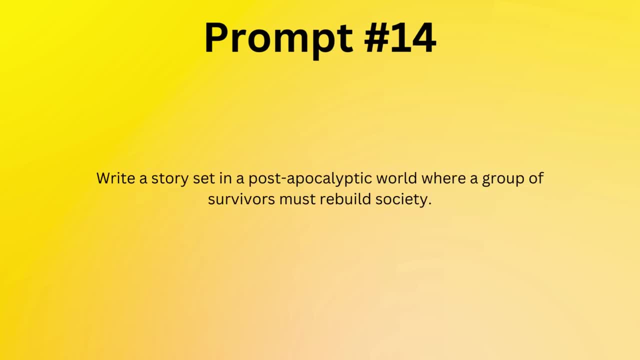 Prompt number fourteen: Write a story set in a post-apocalyptic world where a group of survivors must rebuild society. Prompt number fifteen: Imagine a world where dreams become reality. Write a narrative about someone who discovers their dreams manifest in the waking world. Prompt number sixteen: Craft a personal essay reflecting on a significant childhood memory. 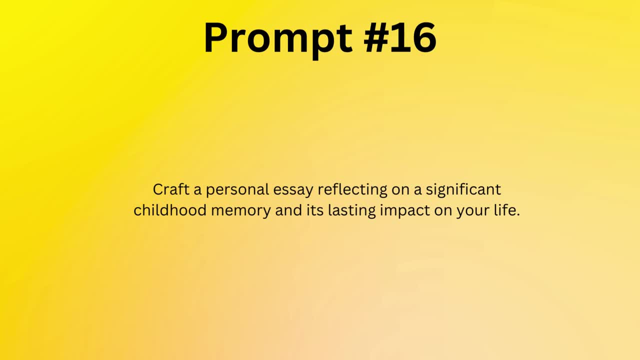 Prompt number seventeen: Write a poem inspired by a natural phenomenon such as a thunderstorm, sunset or blooming flower. Prompt number eighteen: Explore the theme of forgiveness in a short story focusing on a character's journey towards letting go of resentment.